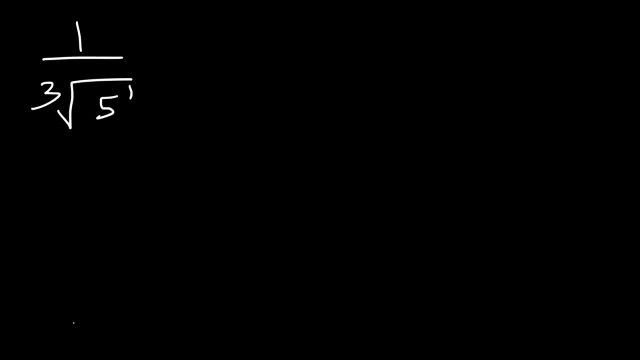 Because the index number is a 3, we need a total of 3 5s on the bottom. Right now we only have one 5, so we need to add two more 5s to it. 5 to the first power times 5 to the second power is 5 to the third power. 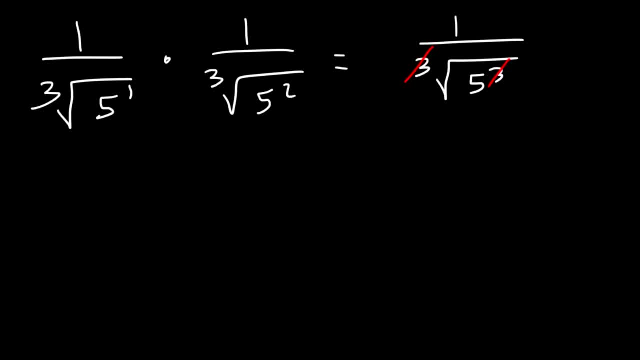 And now these will cancel. and so, Oh, by the way, we need to multiply the top and the bottom, And the bottom by 5 squared. So let me put that here. This is a very important step. So this is going to be the cube root of 25 on top. 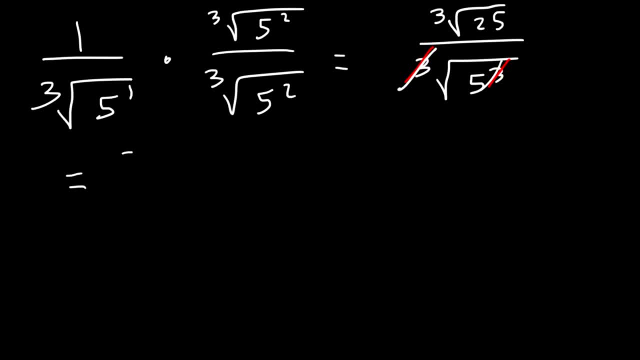 And the 3s will cancel. So on the bottom it's just going to be 5.. So that's the answer. Let's try another example like that. So let's say it's 4 times the cube root of 2.. 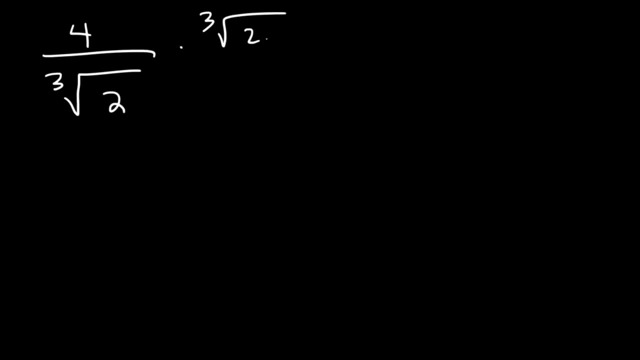 So we need to multiply the top and the bottom by the cube root of 2 squared So we can get a total of 3: 2s on the bottom, 2 squared is 4.. And on the bottom it's going to be 1 plus 2, which is 2 to the third. 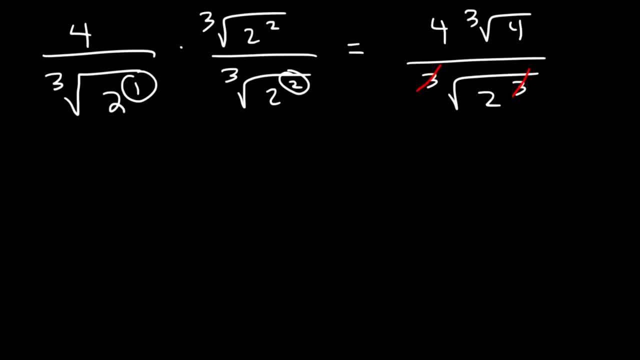 So we need to multiply the top and the bottom by the cube root of 2.. The cube root of 2 to the 3rd, or the cube root of 8, is simply 2.. So this is 4 times the cube root of 4, divided by 2.. 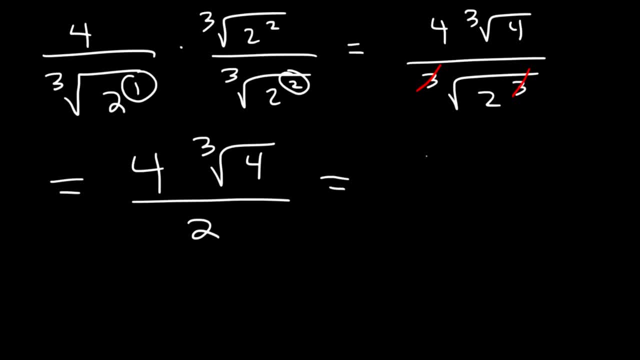 And then we could simplify that 4 divided by 2 is 2, so it's 2 cube root 4.. Let's try this. Let's simplify the cube root of 3 over 4.. So first let's break it into two radicals. 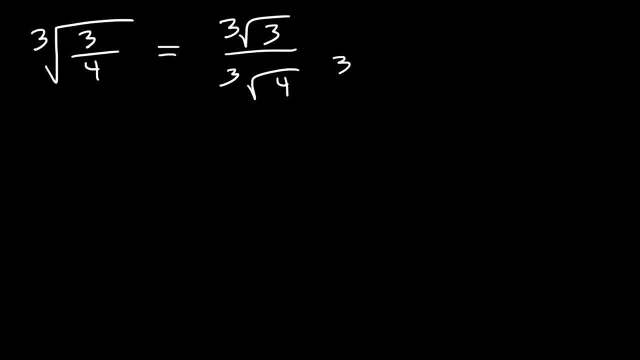 And our goal is to rationalize the denominator. So let's multiply the top and the bottom by the cube root of 4 squared, So we can get three 4's in the bottom. 4 squared is 16. And on the bottom we're going to have the cube root of 4 cubed. 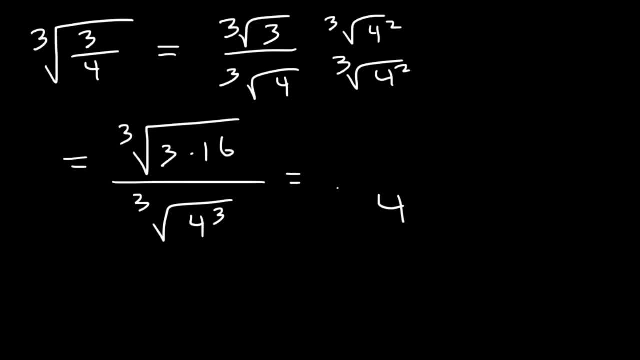 Okay, Which is going to turn into a 4. And 3 times 16 is 48.. So the final answer is the cube root of 48, divided by 4.. Try this one: 3 divided by the cube root of 2y. 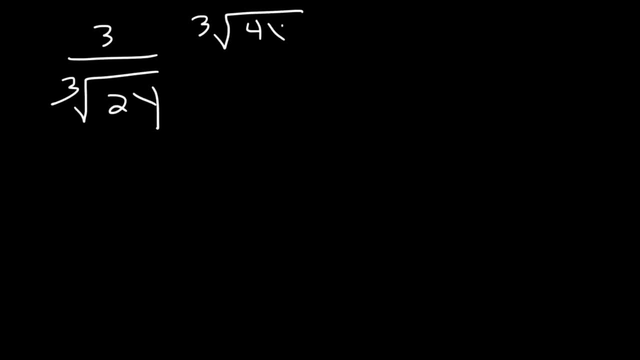 So we're going to multiply the top and the bottom by the cube root of 4y squared. So this is what we're going to have on top. On the bottom: 2 times 4 is 8.. Y times y squared is y cubed. 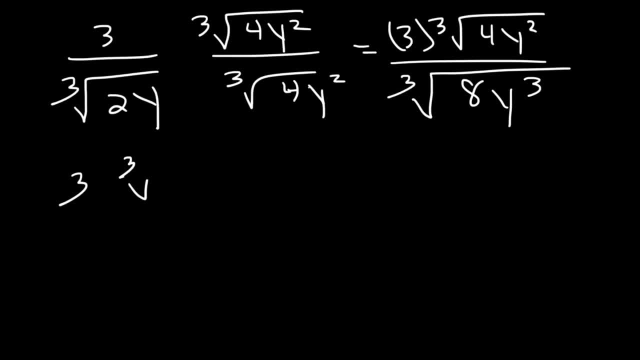 The cube root of 8 is 2.. And the cube root of y cubed is y, And so that's the solution. What about this one 2 times the 4th root of 3x squared? Go ahead and simplify. 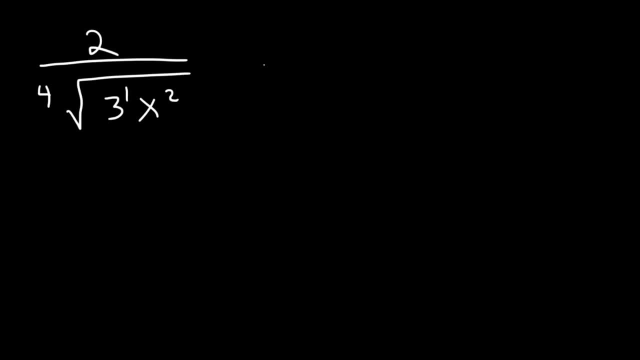 So we need a total of 4 3's and 4 x's. So we need to multiply by 3 to the 3rd. 1 plus 3 is 4, and x squared 3 to the 3rd is 27.. 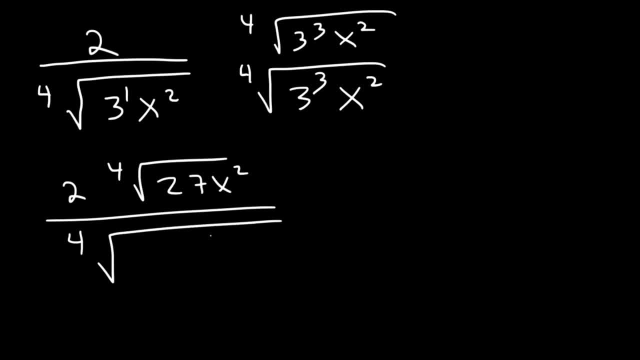 On the bottom, we're going to have 4 3's and 4 x values. So the final answer is 2, 4th root, 27 x squared divided by 3x, where the x is going to be inside an absolute value. 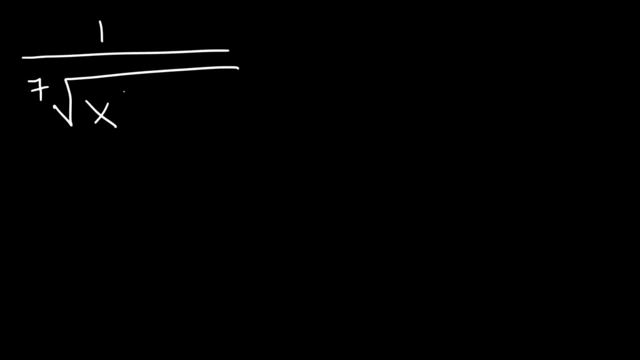 Now what about this example? The 7th root of x squared Y cubed Times z to the 4th. Go ahead and rationalize the denominator, So we're going to have to multiply the top and the bottom by the 7th root of x to the. 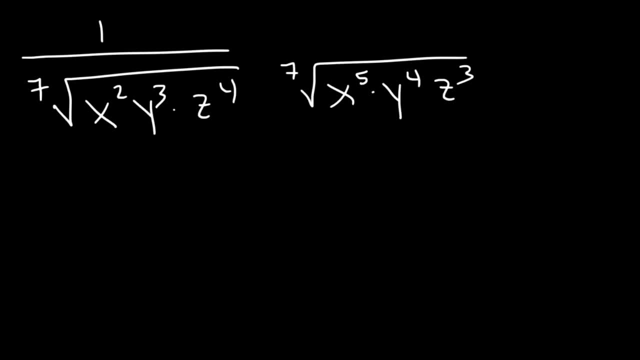 5th y to the 4th, z to the 3rd. We want the exponents to add up to 7.. So on top it's just going to be the 7th root of x to the 5th, y to the 4th. 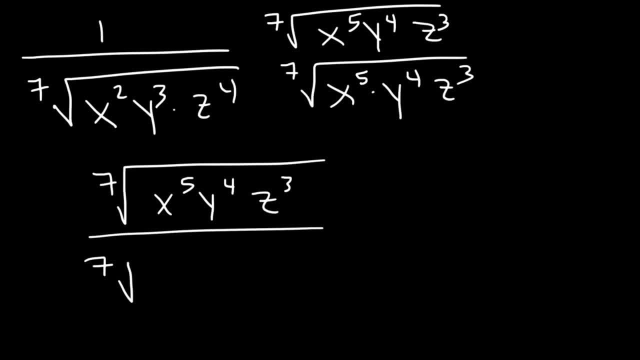 z to the 3rd. On the bottom we have the 7th root of x to the 7th. 2 plus 5 is 7,, 3 plus 4 is also 7, and 4 plus 3 is 7.. 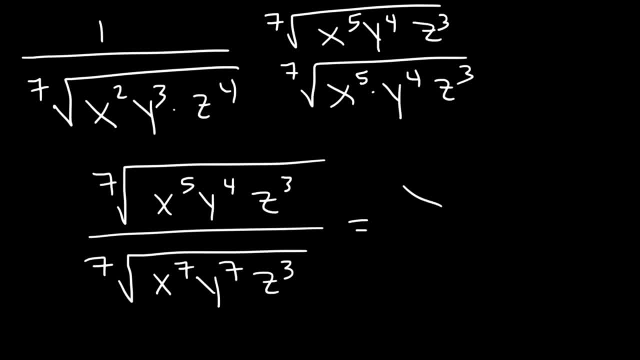 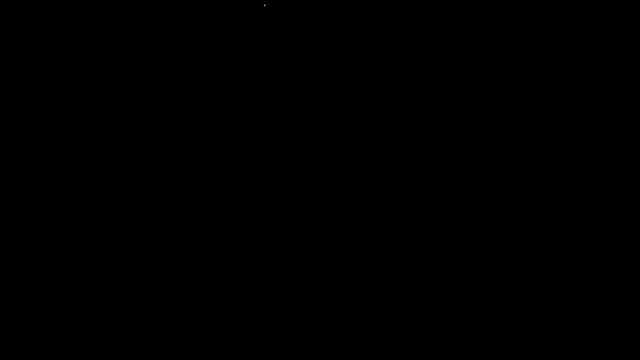 So this is going to be The 7th root of x to the 5th, y to the 4th, z to the 3rd, All divided by x, y, z. What about this one? Go ahead and rationalize the denominator. 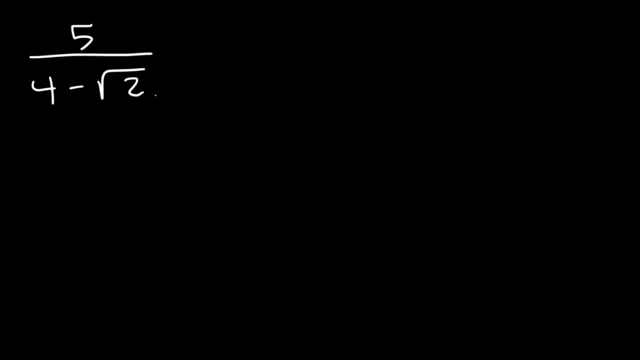 Get rid of all radicals on the bottom. So how can we do that? The only way to get rid of a radical whenever you have two terms is to multiply the top and the bottom by the conjugate. So the conjugate of 4 minus root 2 is 4 plus root 2.. 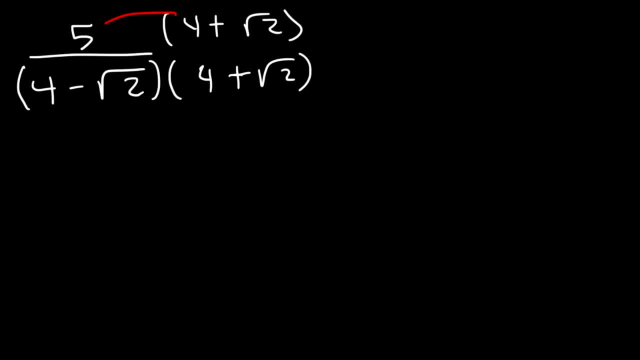 So, on the top, we're going to distribute the 5.. 5 times 4 is 20, and 5 times root 2 is just going to be 5 root 2.. On the bottom, we're going to FOIL. 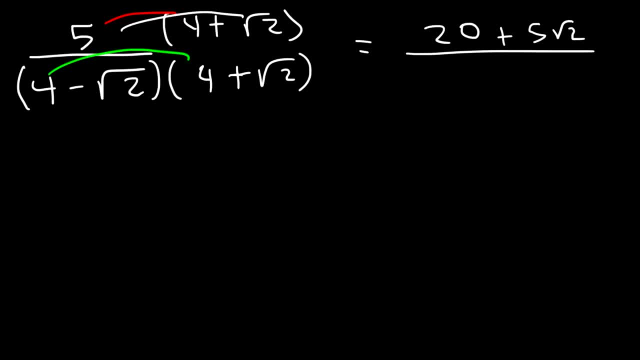 The two middle terms will cancel. Four times 4 is 16.. Four times root 2 is 16.. That's just going to be 4 root 2.. And then negative root 2 times 4, that's negative 4 root 2.. 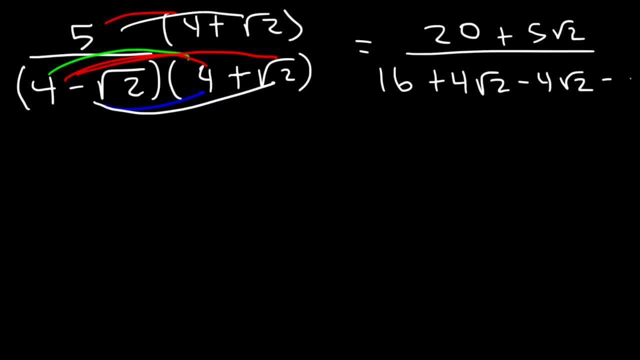 And then finally negative root 2 times root 2 is going to be just negative 2.. So these will cancel, And 16 minus 2 is 14.. So this is the answer. As you can see, there are no more radicals in the denominator of the fraction. 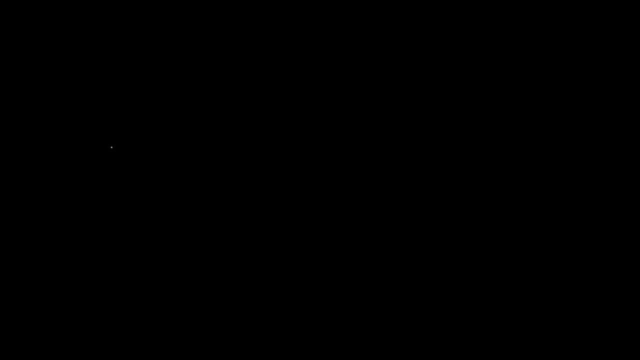 So we're going to get rid of all radicals. So we're going to get rid of all radicals. Here's another example: Go ahead and rationalize the denominator, So we're going to have to multiply the top and the bottom by 4 minus root 3..